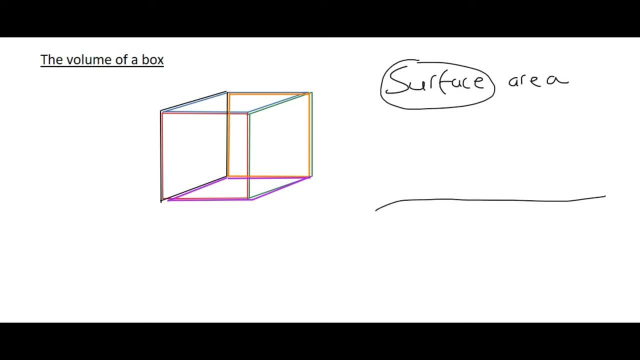 for example, if you have the ocean. so here's a side view of the ocean, with all the little fish swimming beneath. Well, the surface is the part at the top, so it's on the outside. Okay, so, and then area. well, we know what area means. For example, if you have a shape like that, then the area is all. 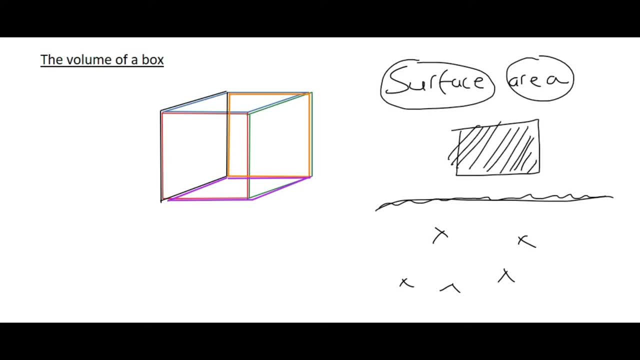 of this over here. So what you do with surface area- and we saw this in the previous video- is you would add up or you would go look at the areas of each part of the shape and then you would just add up all the areas at the end. Now we're looking at something completely different. We are looking at 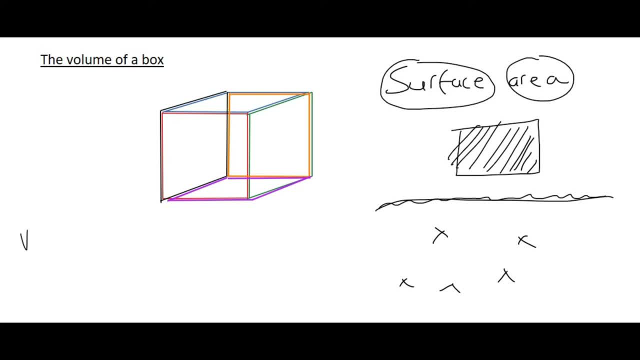 the volume of the box. So we're going to look at the volume of the box. So we're going to look at volume. Okay, so when you think of the word volume, for most shapes you're just going to think of it as area of the base times, height. Okay, so for most shapes, you can think of it. 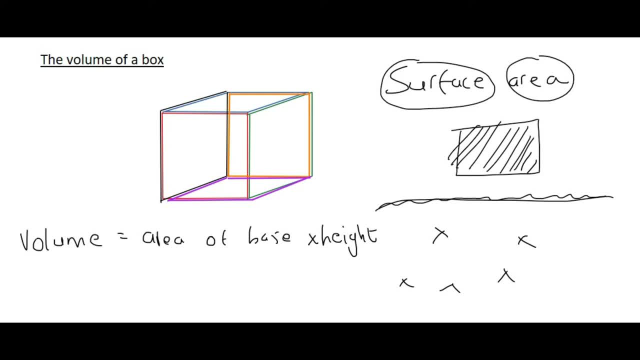 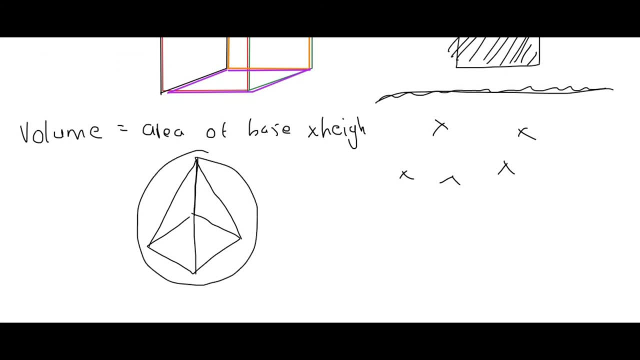 like that. The only time that that will change is when we are busy with pyramid kind of shapes. So any shape that does something like this, where it starts off at the bottom as a square, for example, and then it goes inwards to become a single point at the top. 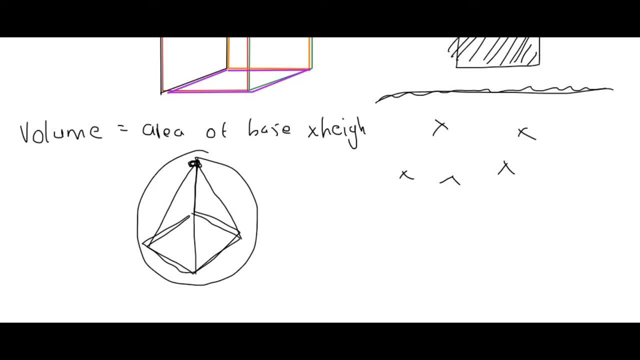 So even a cone is classified. we can classify it as a pyramid. So here's a cone, So notice how the base is round at the bottom, like that, and then it goes inwards to become a point. So when we get a shape like that, then we're going to modify this volume formula and we're simply going to well. 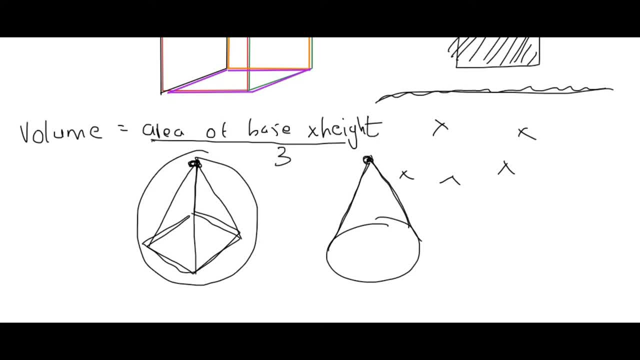 we'll end up having to divide by three, but we'll get to that in later videos, So for now, all I want you to do is think of the following: Volume is equal to the area of the base times by the height. So let's get started. So what you've got to do is you've got to look at the shape and 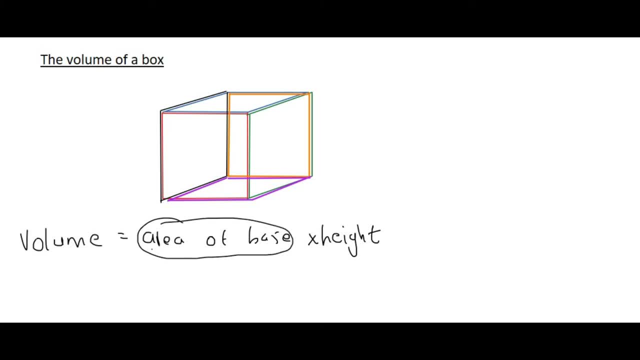 you've got to pick a base. Okay so a base is like a starting point. So let me give some letters over here. Okay so you need to choose yourself a base. So let's say we choose, oh, and then we need one. 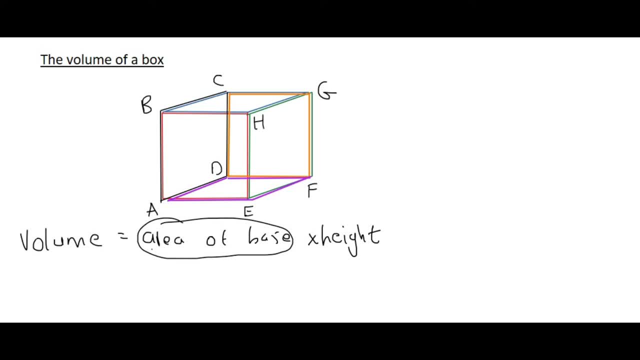 more letter. So let's call this corner letter H. So let's choose. well, let's say, for example, we choose this red square as our base, So we would go work out the area. Now we know how to do the area of that. Let's say it was a rectangle, for example, or a square, And 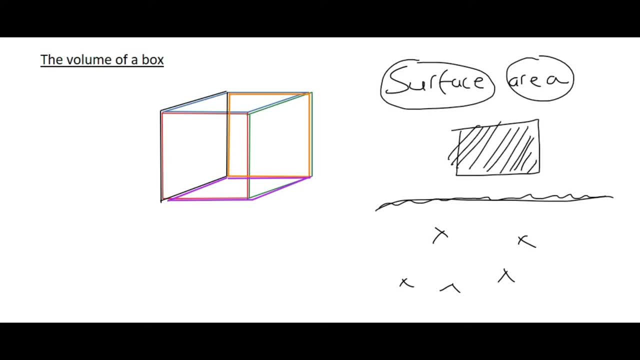 of this over here. So what you do with surface area- and we saw this in the previous video- is you would add up or you would go look at the areas of each part of the shape and then you would just add up all the areas at the end. Now we're looking at something completely different. We are looking at 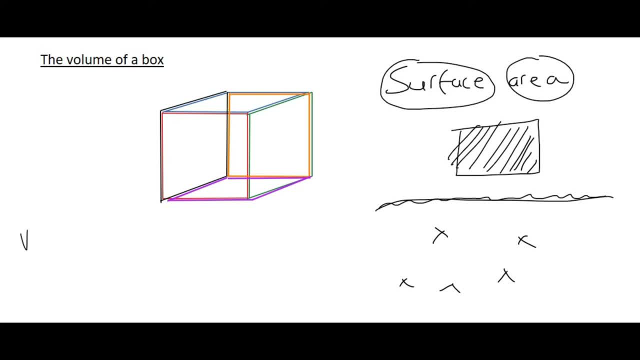 the volume of the box. So we're going to look at the volume of the box. So we're going to look at volume. Okay, so when you think of the word volume, for most shapes you're just going to think of it as area of the base times, height. Okay, so for most shapes, you can think of it. 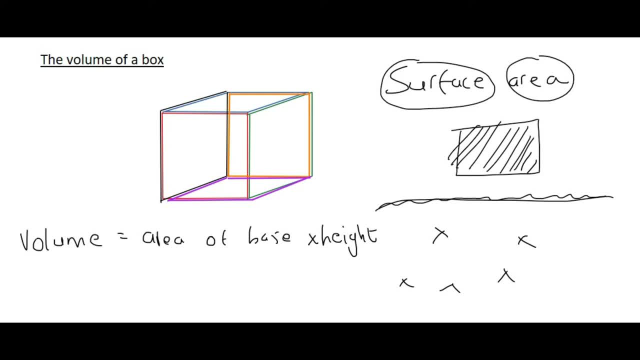 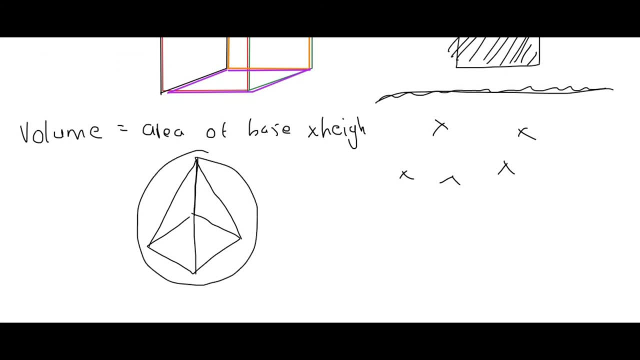 like that. The only time that that will change is when we are busy with pyramid kind of shapes. So any shape that does something like this, where it starts off at the bottom as a square, for example, and then it goes inwards to become a single point at the top. 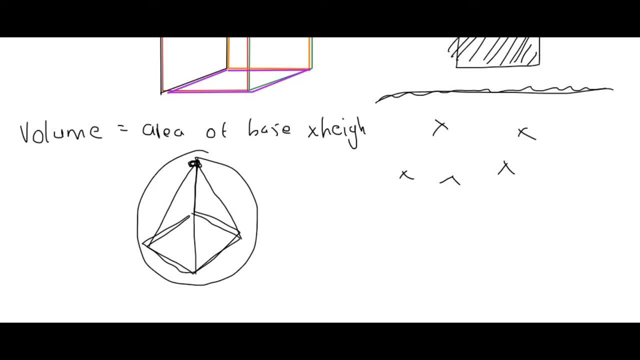 So even a cone is classified. we can classify it as a pyramid. So here's a cone, So notice how the base is round at the bottom, like that, and then it goes inwards to become a point. So when we get a shape like that, then we're going to modify this volume formula and we're simply going to well. 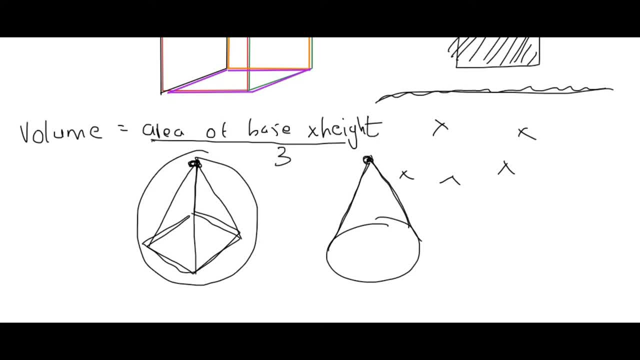 we'll end up having to divide by three, but we'll get to that in later videos, So for now, all I want you to do is think of the following: Volume is equal to the area of the base times by the height. So let's get started. So what you've got to do is you've got to look at the shape and 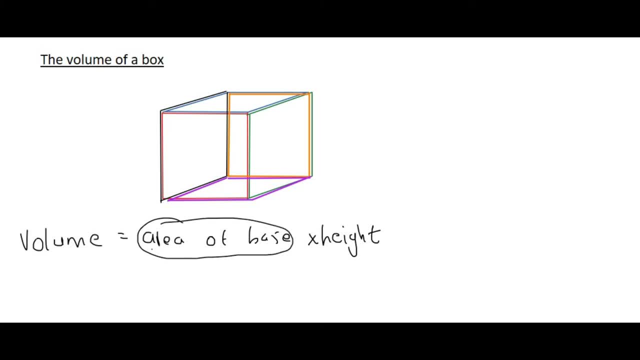 you've got to pick a base. Okay so a base is like a starting point. So let me give some letters over here. Okay so you need to choose yourself a base. So let's say we choose, oh, and then we need one. 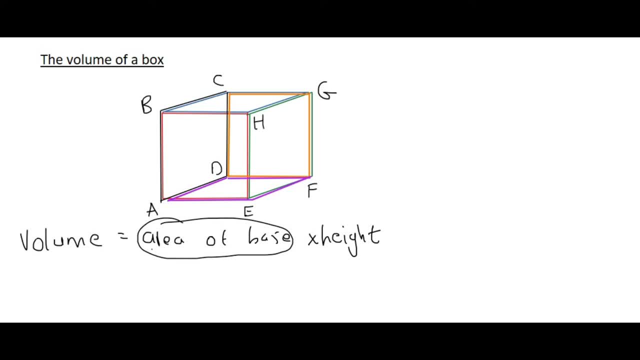 more letter. So let's call this corner letter H. So let's choose. well, let's say, for example, we choose this red square as our base, So we would go work out the area. Now we know how to do the area of that. Let's say it was a rectangle, for example, or a square, And 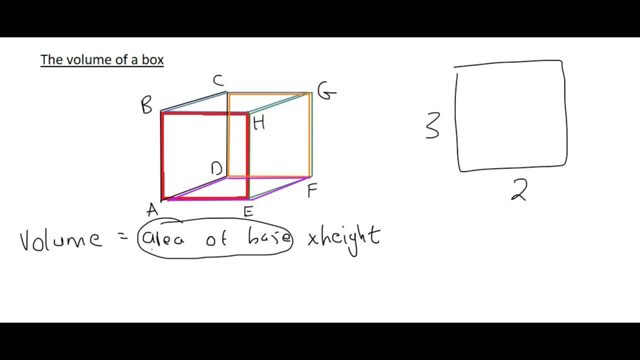 so let's choose a rectangle. So let's say this length was three and this length was two. Well, to work out the area, that's just three times two, right? So that would be six. Now, okay, so we've done the area of the base. Then we need to look at the height. So imagine you could take 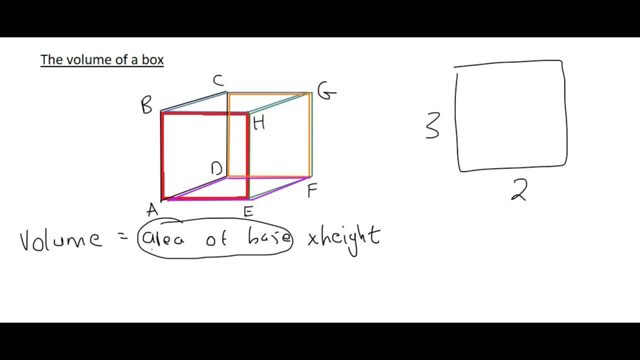 so let's choose a rectangle. So let's say this length was three and this length was two. Well, to work out the area, that's just three times two, right? So that would be six. Now, okay, so we've done the area of the base. Then we need to look at the height. So imagine you could take 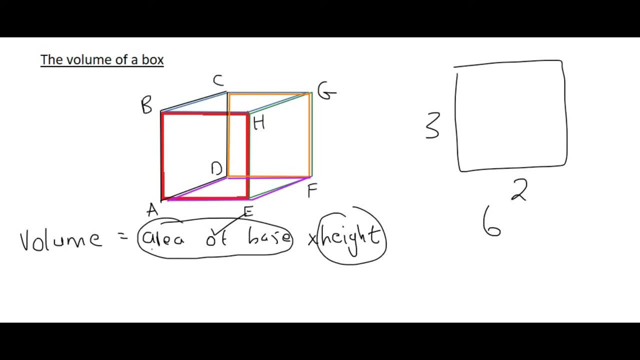 that red square. Now, how would you have to drag that red square so that it completes the whole shape? Okay, so I've gone and I've just colored in that first red square. Now we would have to all the way to the back, because imagine you had to drag it all the way to the back. Well, 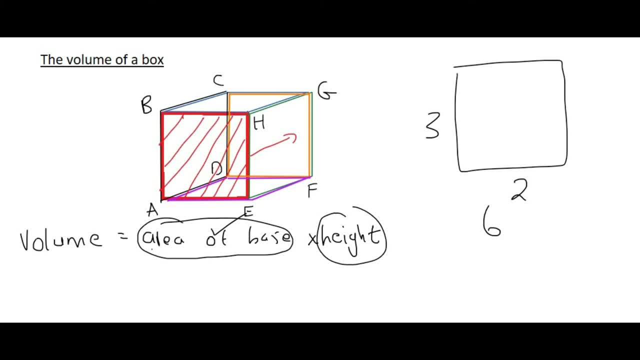 then it would complete the entire shape of the box, And so that is what we mean by the height. So the height is going to be the distance from E to F, or from H to G or from B to C, for example. 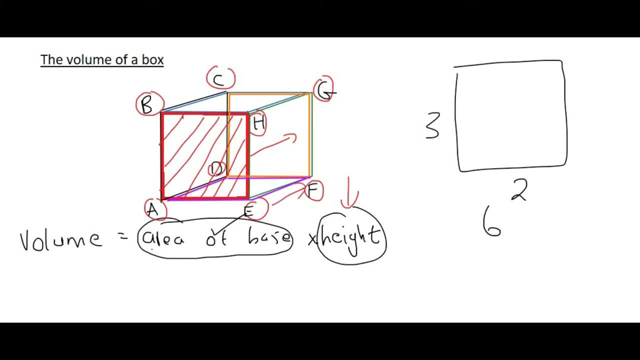 or from A to D, So you'd have to drag it in that direction over there. So let's say the distance from E to F was four, So then your area of your base is six, And so you'd have to drag it in that. 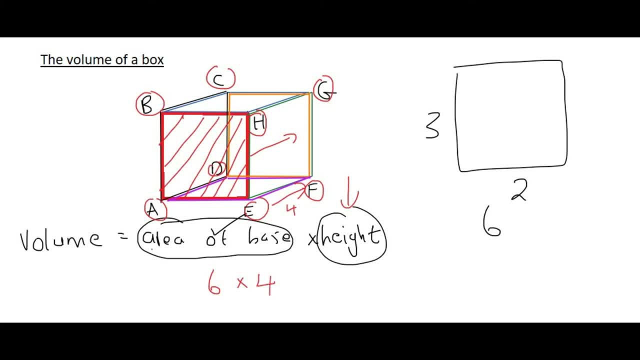 times your height, which we're going to call four. Let's do it in a different way. Let's say we chose the green side as our base, So then you would go work out the area of. so, if the green side's your base, you would go work out that area, which is very easy to do. It's just a rectangle, or. 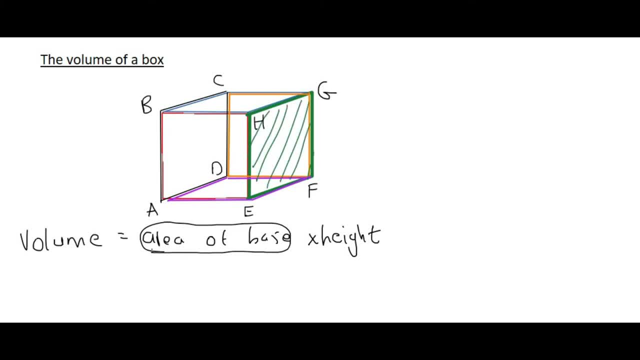 a square. Then how? and then let me quickly color in that base- Then how would you have to drag that shape, that green block? How would you drag that so that it completes what fills up the entire shape? Well, you would now have to do that, So you would have to drag that shape, that green block. 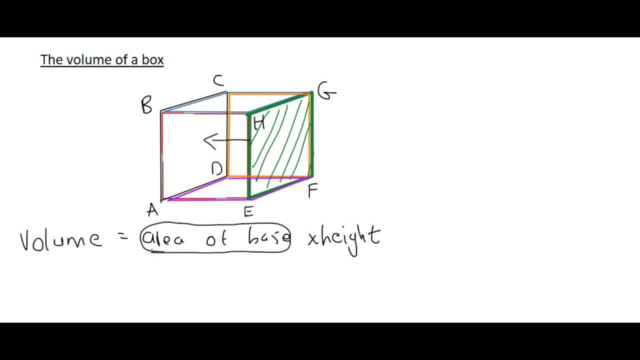 in that direction. Imagine sliding that green block across, And every time you slide it it fills up more and more of the shape. So, for example, once you get to the halfway point, it would look like this: See, so notice, we've now completed half of the shape. And then we would continue dragging in. 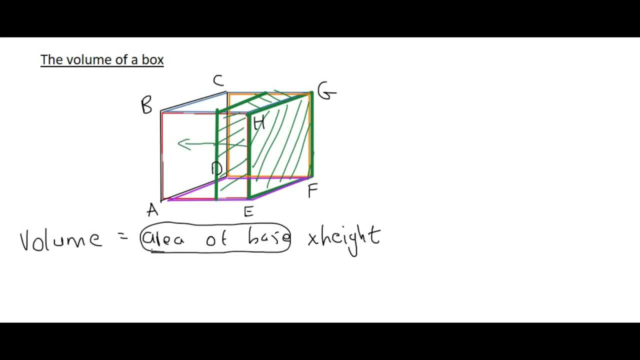 that direction And eventually you would reach the very end, And that would be called the height. Okay, so you choose a base and then you drag that base until it completes the shape, And that means that you have to drag it, which in this example, would be from E to A. that would be called. 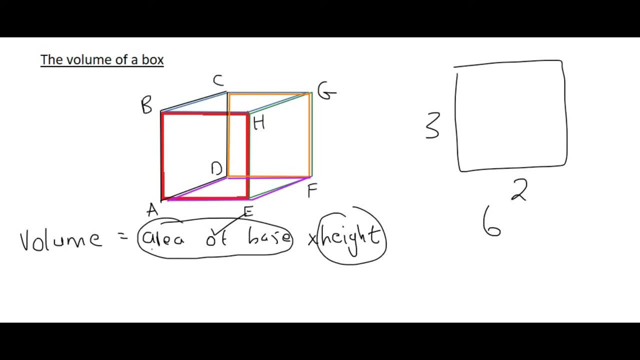 that red square. Now, how would you have to drag that red square so that it completes the whole shape? Okay, so I've gone and I've just colored in that first red square. Now we would have to all the way to the back, because imagine you had to drag it all the way to the back. Well, 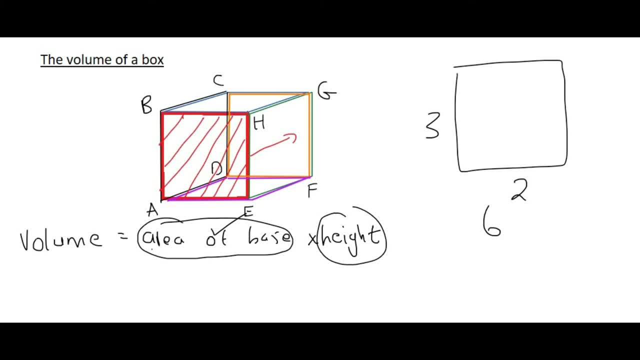 then it would complete the entire shape of the box, And so that is what we mean by the height. So the height is going to be the distance from E to F, or from H to G or from B to C, for example. 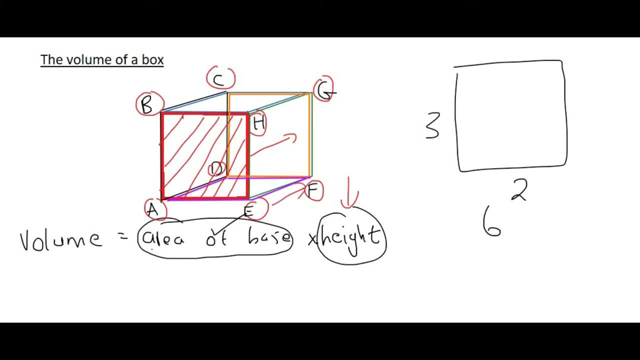 or from A to D, So you'd have to drag it in that direction over there. So let's say the distance from E to F was four, So then your area of your base is six, And so you'd have to drag it in that. 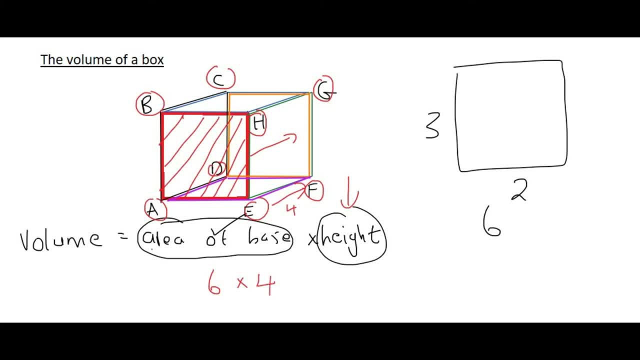 times your height, which we're going to call four. Let's do it in a different way. Let's say we chose the green side as our base, So then you would go work out the area of. so, if the green side's your base, you would go work out that area, which is very easy to do. It's just a rectangle, or. 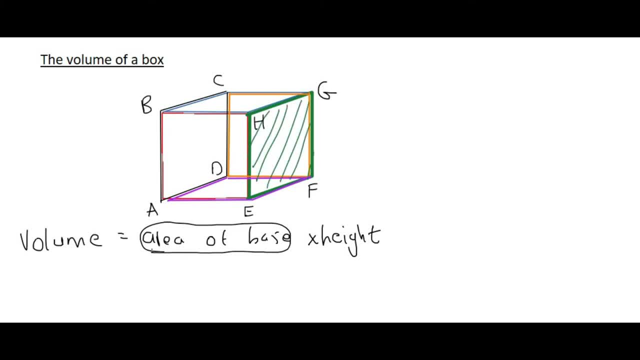 a square. Then how? and then let me quickly color in that base- Then how would you have to drag that shape, that green block? How would you drag that so that it completes what fills up the entire shape? Well, you would now have to do that, So you would have to drag that shape, that green block. 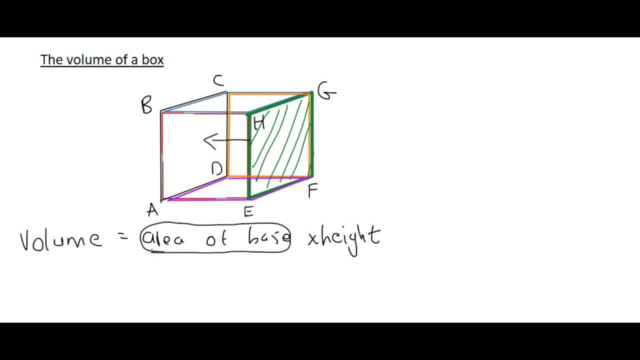 in that direction. Imagine sliding that green block across, And every time you slide it it fills up more and more of the shape. So, for example, once you get to the halfway point, it would look like this: See, so notice, we've now completed half of the shape. And then we would continue dragging in. 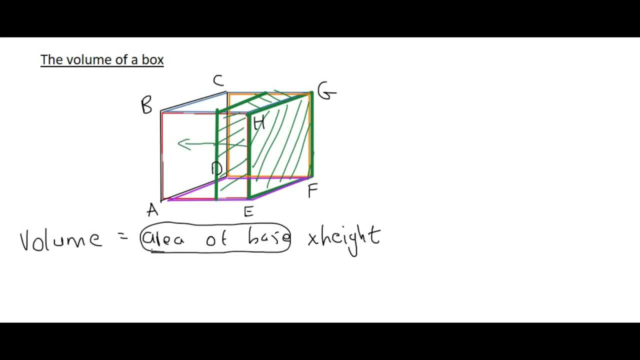 that direction And eventually you would reach the very end, And that would be called the height. Okay, so you choose a base and then you drag that base until it completes the shape, And that means that you have to drag it, which in this example, would be from E to A. that would be called. 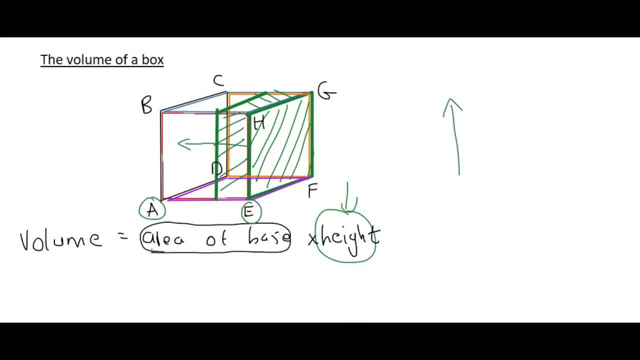 the height. So when we say height, we don't necessarily always mean going up.